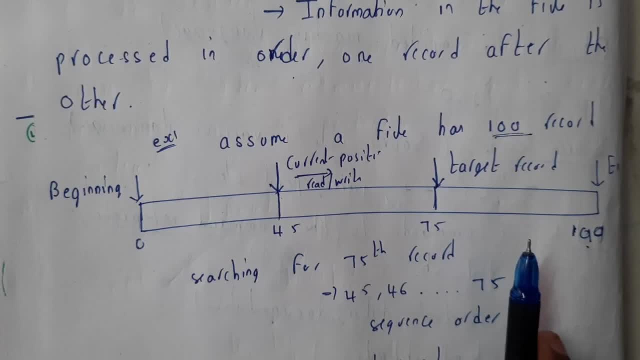 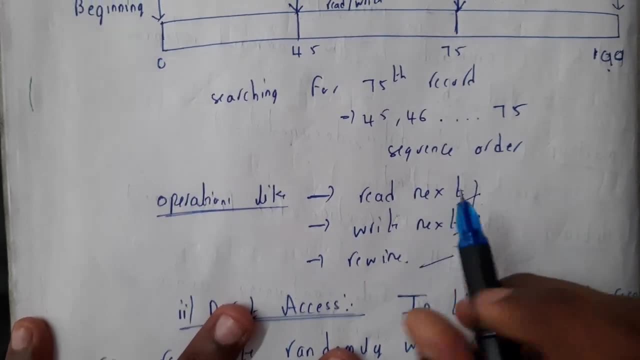 or sequential access is not so quite used nowadays. So basically the operations for this will be read, write and next. So we'll be reading the value: next, next, next, next read, next, read, next, next, next, next, next, like that will be going to the 75th record. 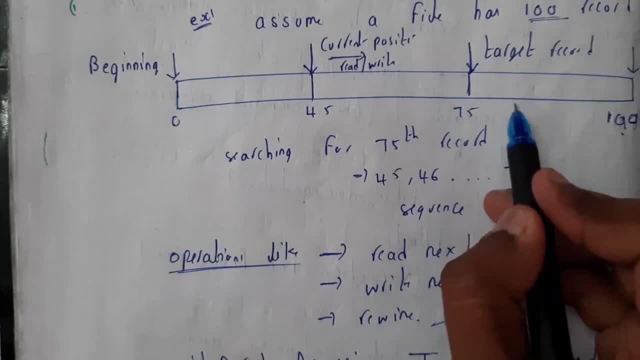 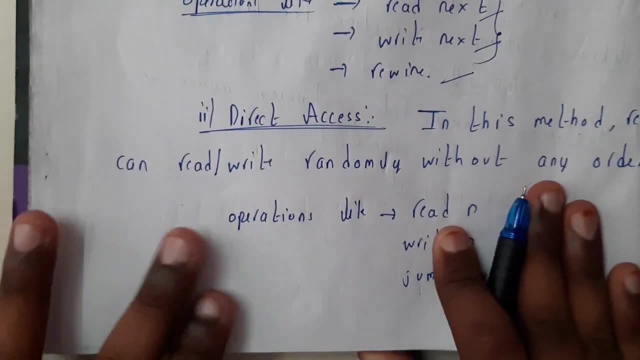 And then you'll be reading it. So, unfortunately, if you are after it, you are at 78 and now you need to come back, So you'll be using rewind, fine, Okay. so now let us go through direct access. So direct access is better than sequential access, guys. So in this method the record can be read, or 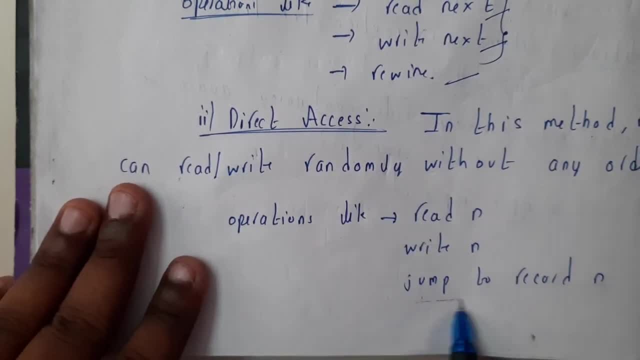 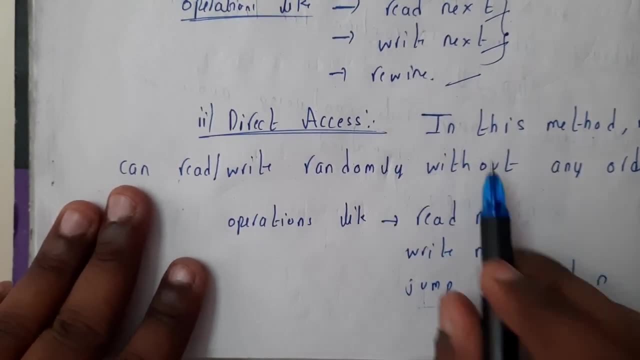 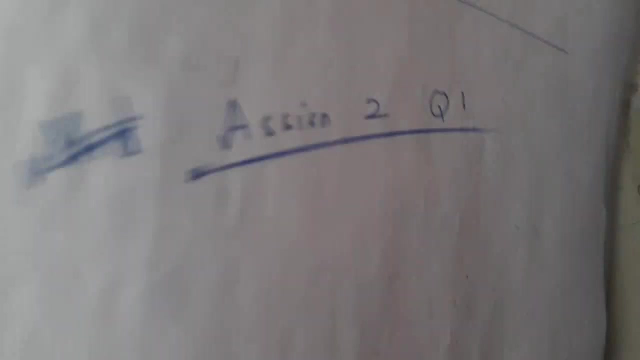 written randomly to that particular location. See here: jump to the record n. So jump to 75th record. You'll be directly jumping to 75th record and you'll be reading it. fine, Okay, so operations read, write and jump to that particular record are available. fine, So, and the last type is index. 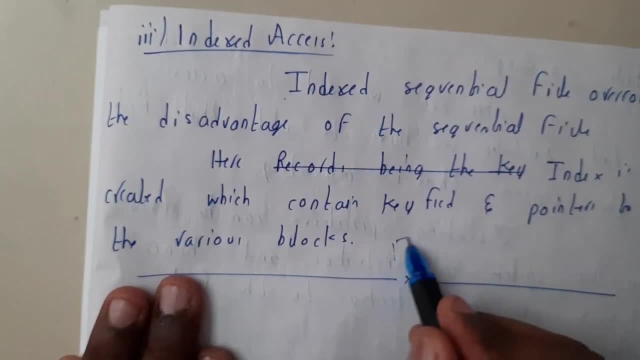 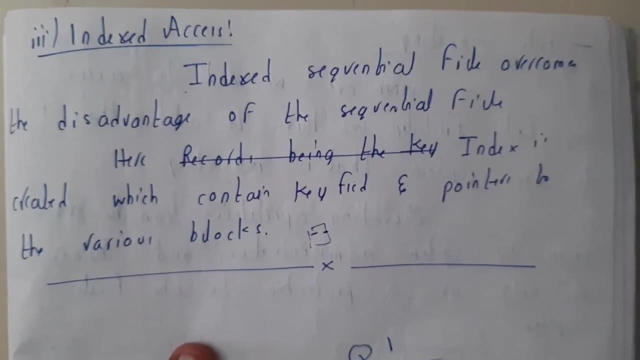 access: indexed access: fine, So indexed. we'll be having a small index with the key field and pointer guys. So according to the key field, you'll be going to that particular pointer and you'll be finding your result there, Like it's just like your index in your classworks or in your printed. 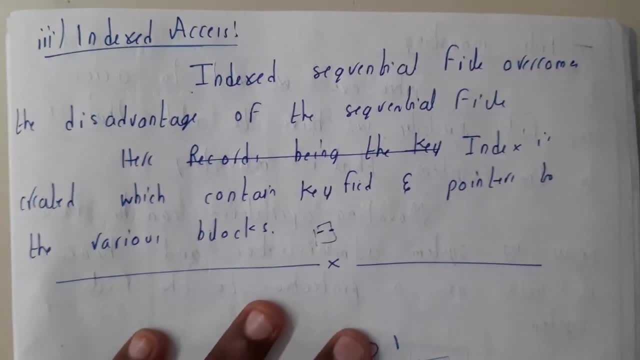 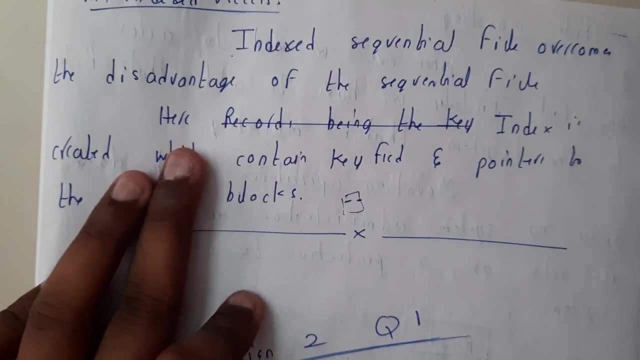 textbooks. fine, So indexed sequential file. it overcomes the sequential problems and disadvantages in the sequential file. So this is the way to do it. So this is the way to do it. So this is the way to do it, guys. So here index is created which contains the key field and pointer to various 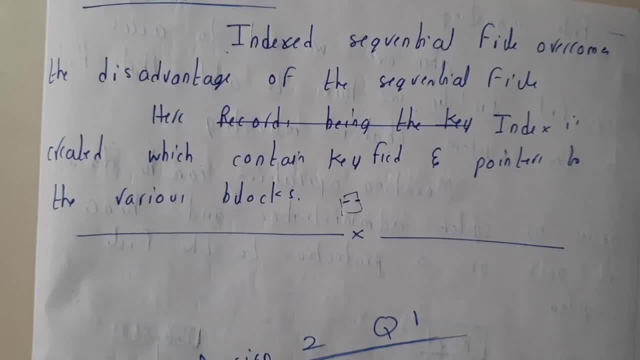 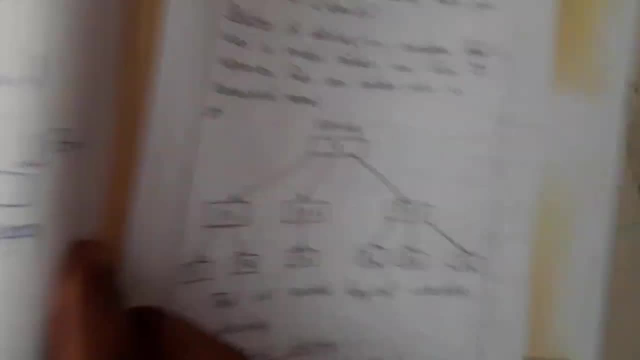 blocks. So using that, we will be accessing them really faster. So I hope everyone got a clear idea on this, guys. So in the next tutorial we will be going through the directories guys. We'll be going through directories introduction and their structures. So let us meet in the next. 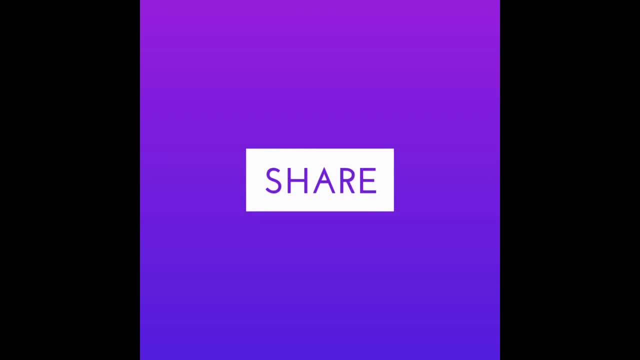 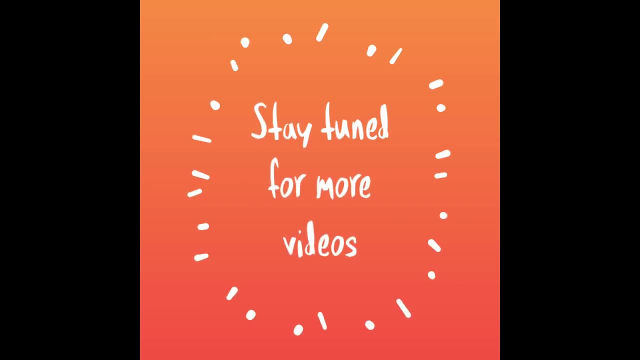 tutorial, Thank you. Thanks for watching Subtitles by the Amaraorg community.